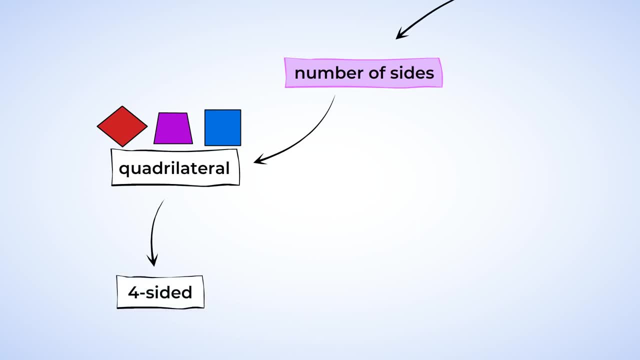 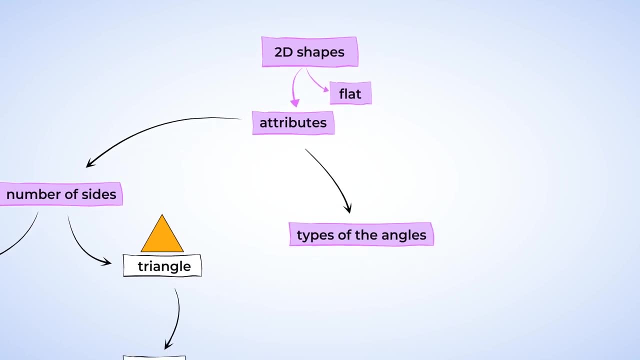 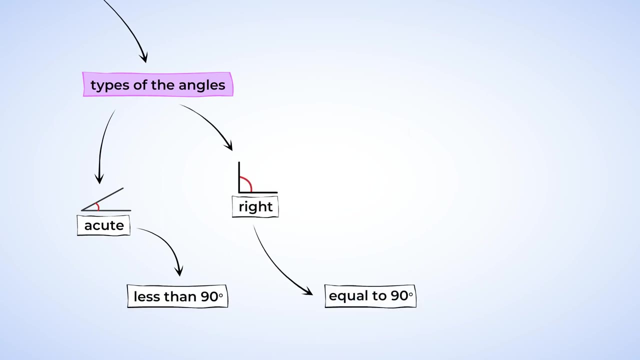 A four-sided figure is called a rectangle, A quadrilateral. A three-sided one is a triangle. right. Another attribute can be the types of the angles. Angles can be classified as acute less than 90 degrees, right equal to 90 degrees, or obtuse greater than 90 degrees. 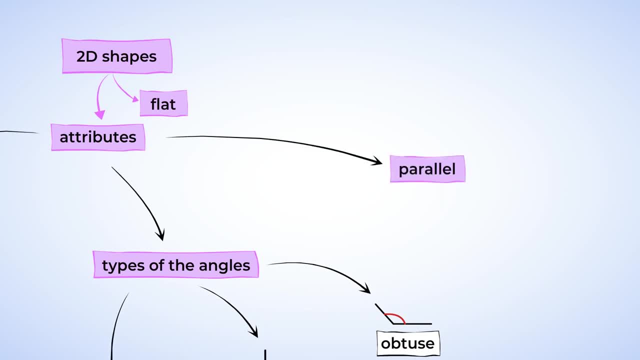 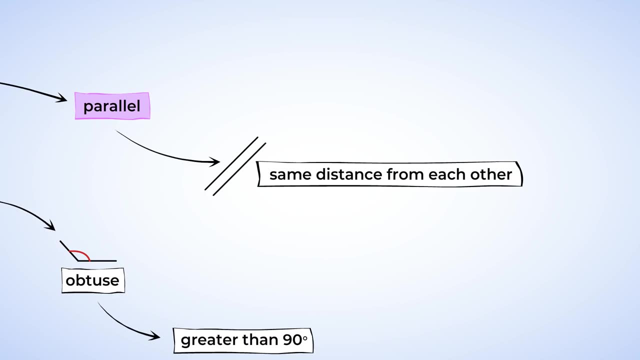 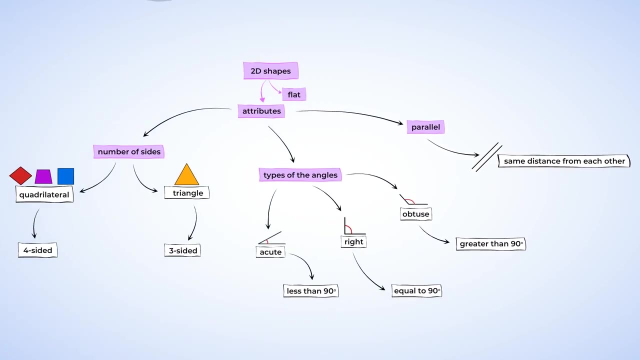 And yet another attribute would be if the sides are parallel. Parallel sides are always the same distance from each other, And if they were extended on till infinity They would never touch. So all those shapes can be organized into different categories, And sometimes they may be part of multiple groups. 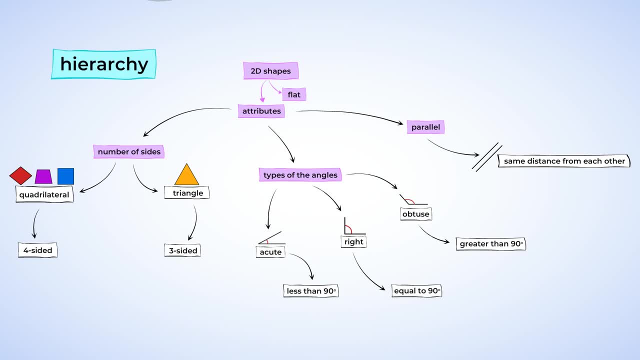 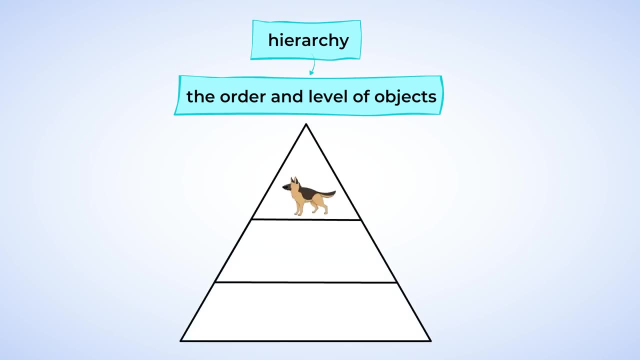 This is called a hierarchy. Yeah, that's a fancy word, but it simply shows the order and level of objects. For example, a German Shepherd is a type of dog. A dog is a type of animal. Now, there are all sorts of different categories. 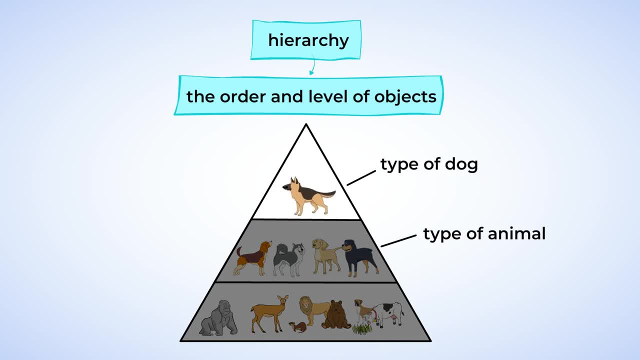 The small one is the type of animal. The small one is the type of animal. The big one is the type of dog- a German Shepherd. The bigger one is the type of animal: dog. Now, those two are called subcategories of the main category: animal. 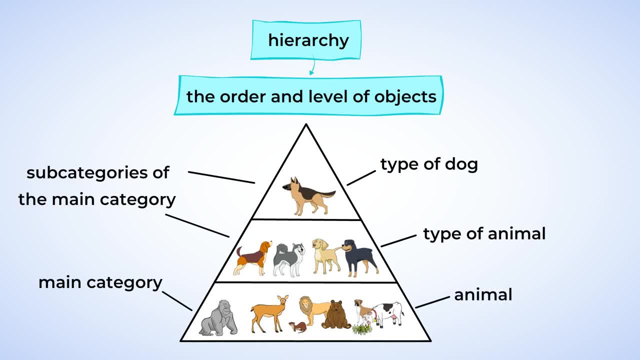 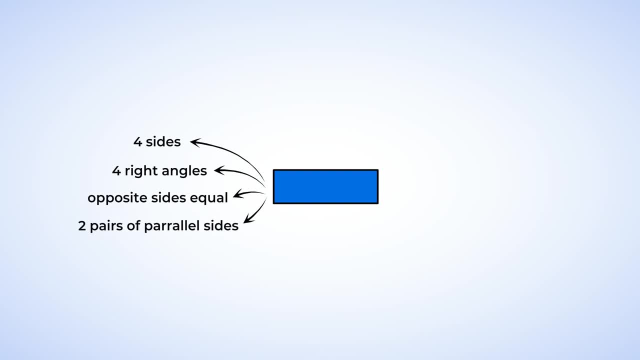 And this is the same with shapes. Let's look at some quadrilaterals. A rectangle is a quadrilateral with four right angles and two sets of parallel sides. This square has those same attributes, So a square is also a type of rectangle. 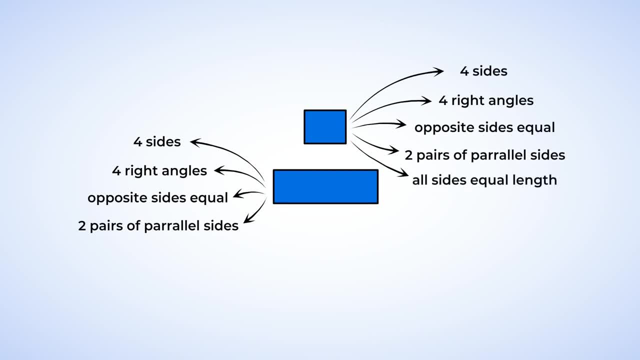 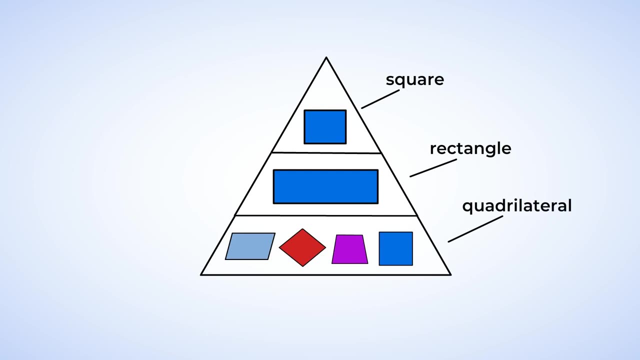 Since a square has four sides that are all the same length, it's a specific type of rectangle And therefore we have the subcategory square, We have the larger category rectangle, Then even larger quadrilaterals, which are part of the main group: polygons. 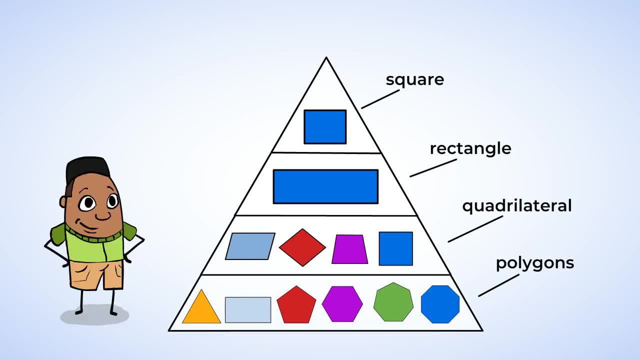 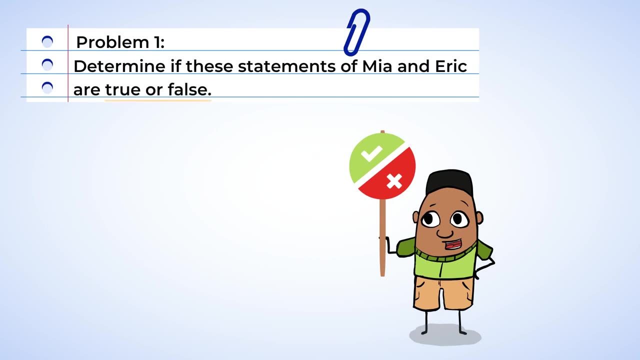 Triangles are part of polygons too, And now that we've reviewed some of the attributes of shapes and their hierarchy, let's see if we can solve some puzzles. Bring them on. Alright cool. True or false statements. Alright, let's determine if these statements are true or false. 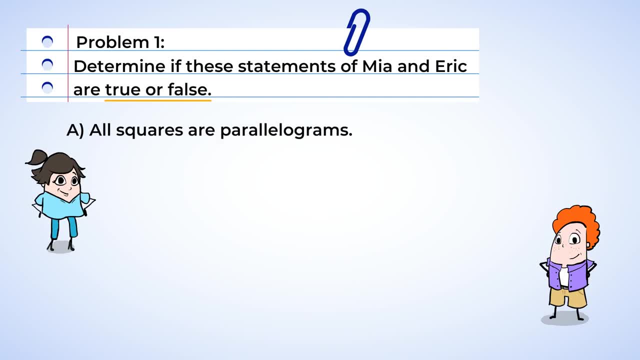 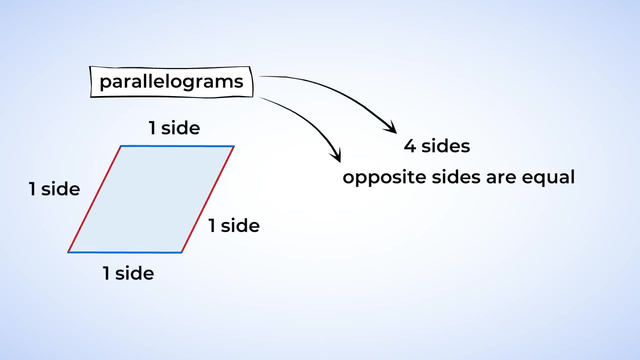 And here we go. Mia claims that all squares are parallelograms. Hmm, well, that might be a new word for you, So let's introduce some useful definitions. A parallelogram is a shape that has four sides, with opposite sides that are the same length and are parallel to each other. 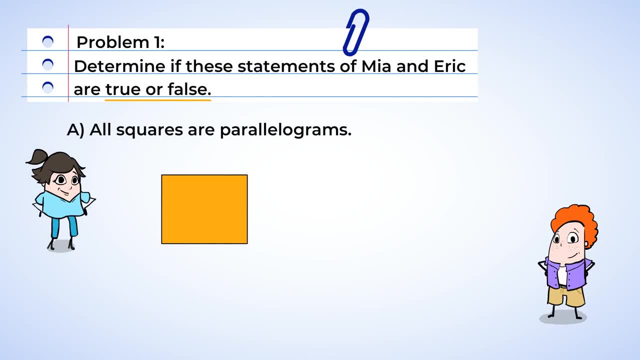 Squares have those attributes as well. Therefore, Mia's statement is true. Okay, and the second statement comes from Eric. He claims that all rectangles are squares. Hmm, does a rectangle have all of the same attributes as squares? They both have four sides and four angles that are 90 degrees. 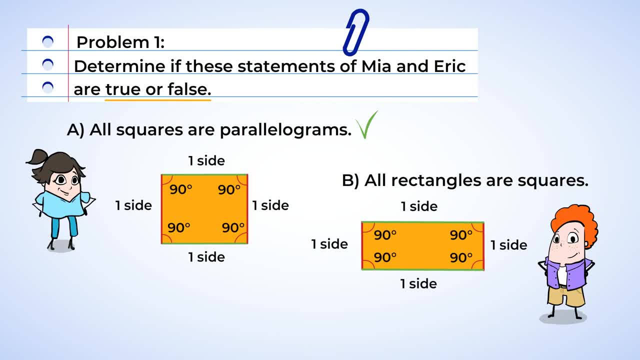 They have opposite sides, They're parallel. A square has four equal sides? Hmm, but equal sides are not necessary attributes for all rectangles. Since a rectangle only has opposite sides that are the same length, it can't be a square, And this means that Eric's statement is false. 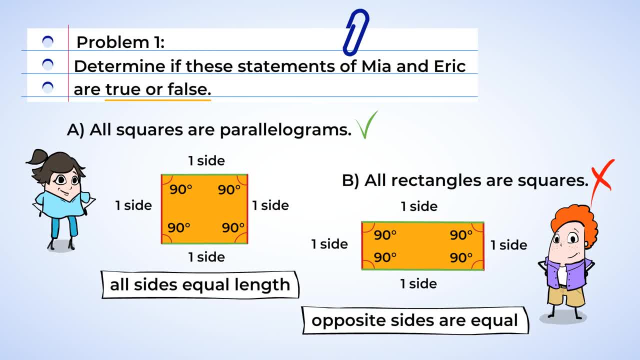 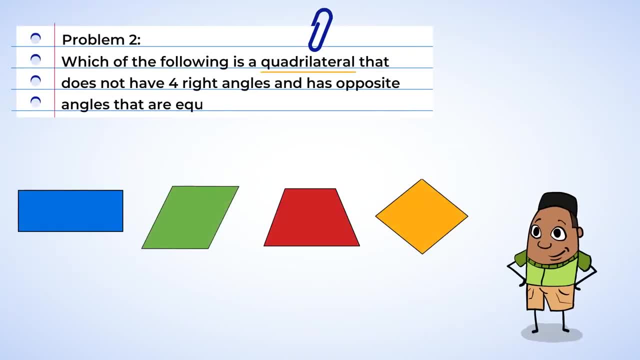 He has it backwards. If he had said all squares are rectangles, then that would have been correct. Now let's see another problem. Which of the following Is a quadrilateral that does not have four right angles and has opposite angles that are equal? 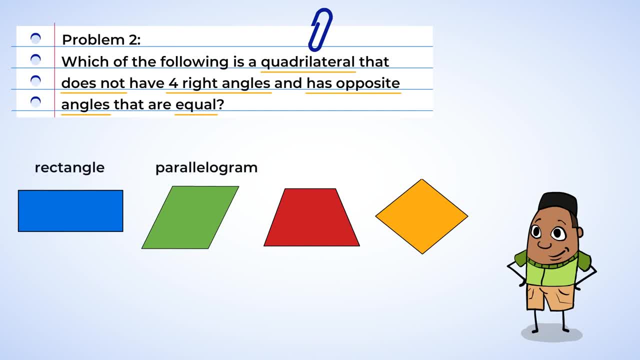 Well, we have the options of a rectangle, a parallelogram, a trapezoid and a rhombus. Well, let's start with the first clue. The shape is a quadrilateral and that means it has four sides. 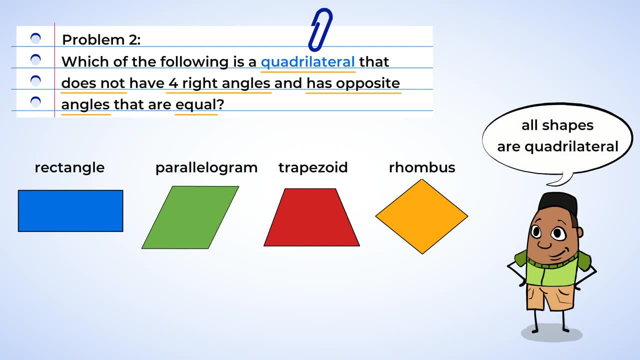 Well, all of these shapes are quadrilaterals, so let's move on to the next clue to see if that'll help us. Does not have four right angles. Well, a rectangle has four right angles, so we can cross that shape off. 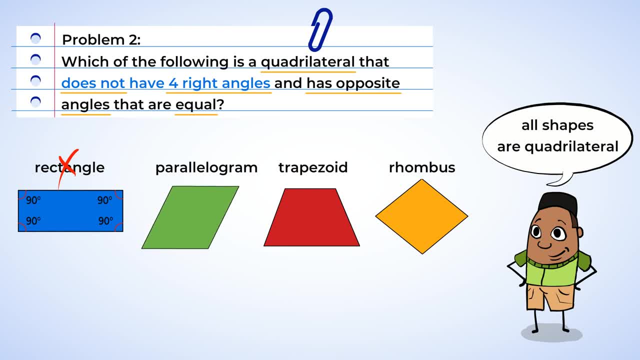 A parallelogram can have four right angles, but it doesn't necessarily have to. We won't cross it off yet. Now for our final clue: opposite angles that are equal. Well, let's take a look at these shapes and their opposite angles. 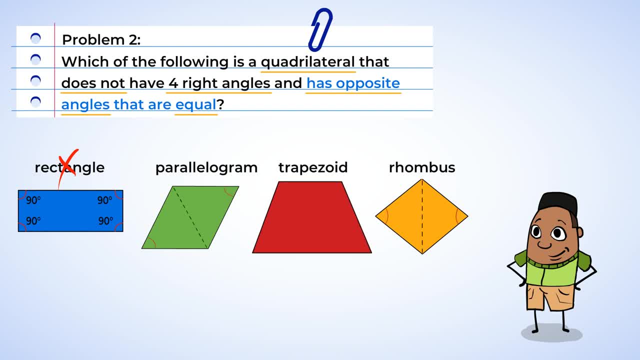 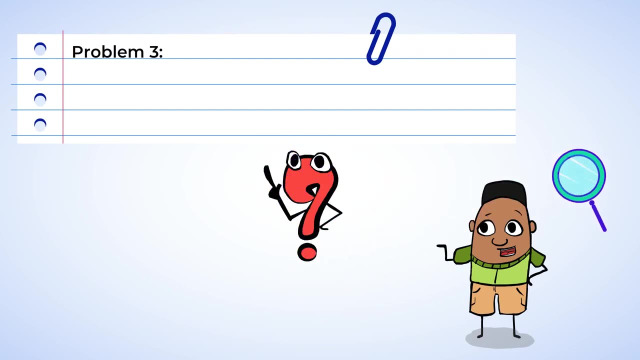 A parallelogram and a rhombus have opposite angles that are equal. A trapezoid does not, Oh, Make this statement true. Parallelogram and rhombus: A riddle. Cool Will has the following riddle: 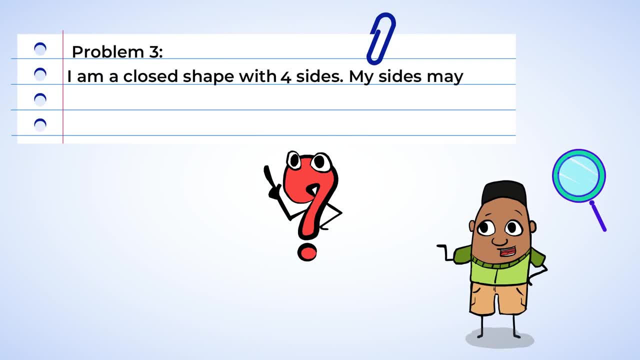 I am a closed shape with four sides. My sides may be the same length or equal length. I do not have any parallel sides and no right angles. What am I? Okay, let's start with the first clue: It's a closed shape with four sides. 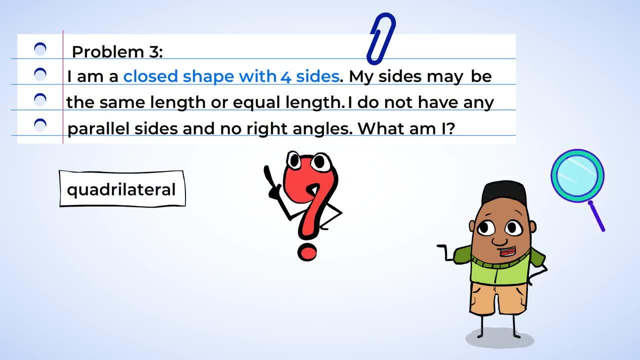 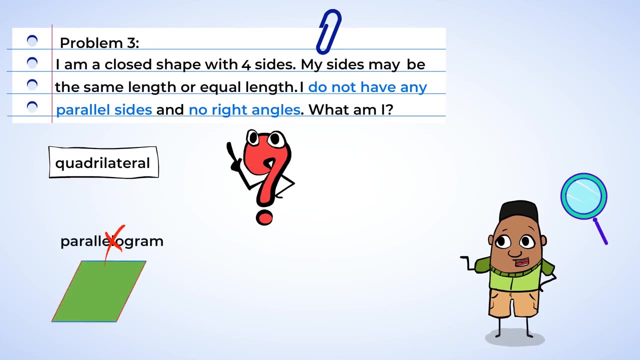 And this means that it's a quadrilateral. Well, the next clue doesn't tell us much, since the sides may or may not have equal lengths, And we also know that there are no parallel sides or right angles, And this means that it can't be a parallelogram or any of the shapes that are specific parallelograms. 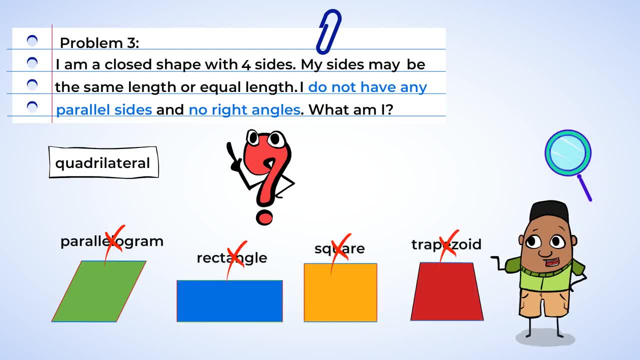 like rectangles or squares, And it also can't be a trapezoid, since those have one pair of parallel sides. Wow, This is a trick. It's a tricky riddle. Good job Will, But no worries, my mighty friend. 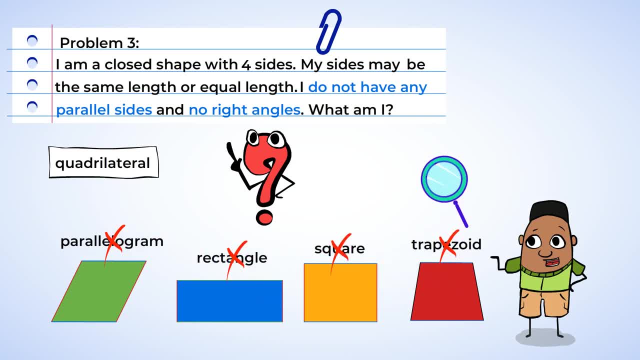 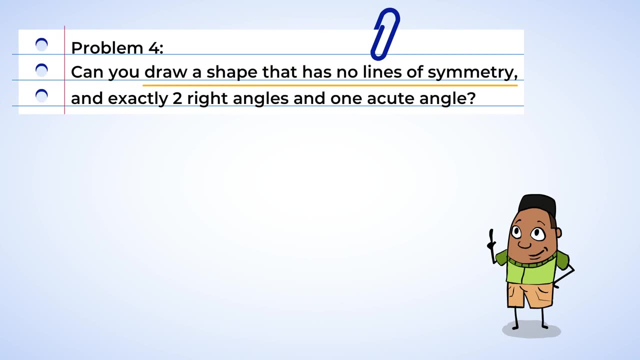 If we can't guess the precise shape or the subcategory of the quadrilateral, we can always say what we know, And we already guessed quadrilateral, which is correct. And the final riddle for today: Can you draw a shape that has no lines of symmetry? exactly two right angles and one. 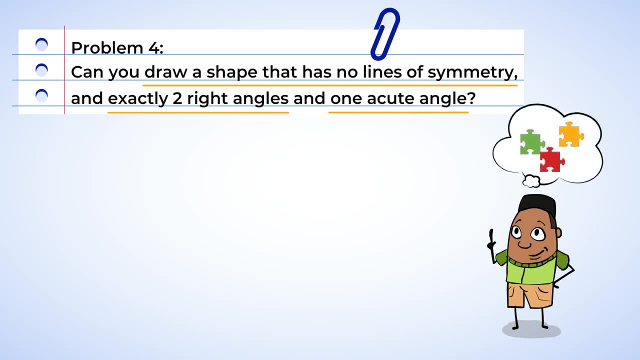 acute angle. Ooh, this sounds like a fun puzzle. Now let's start by drawing the angles. Here are two right angles, and they each have a measure of 90 degrees, And here's an acute angle with a measure smaller than 90 degrees. 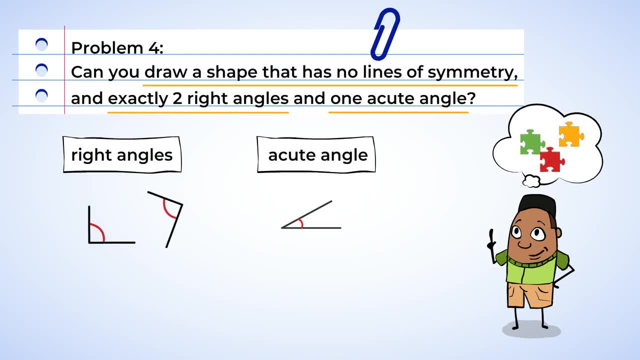 Let's see if we can fit these together. Ooh, and if we move it like that, maybe like that? hmm, a shape that has three angles is a triangle. When we make two of the angles in the triangle 90 degrees, 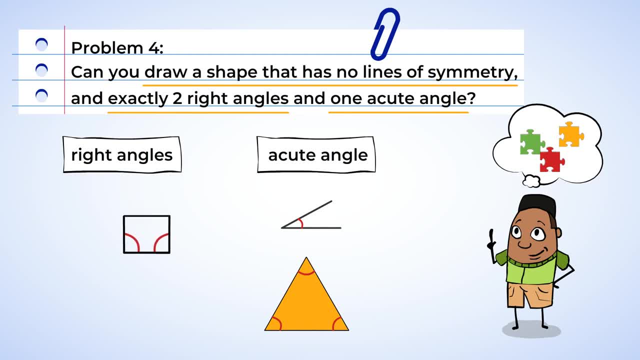 There's a gap If we create a line to close, the shape in it no longer has three angles. I think this shape is impossible to make. So the answer is no, we can't draw a shape like that. It's mission impossible. 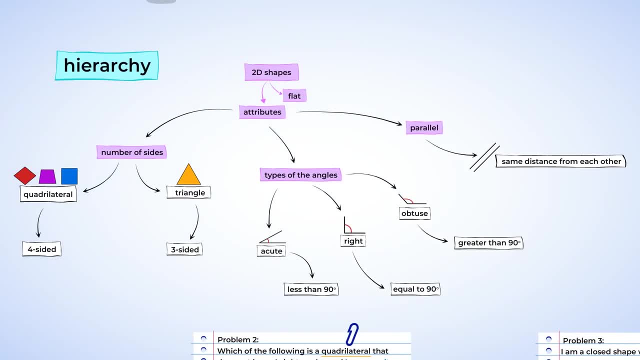 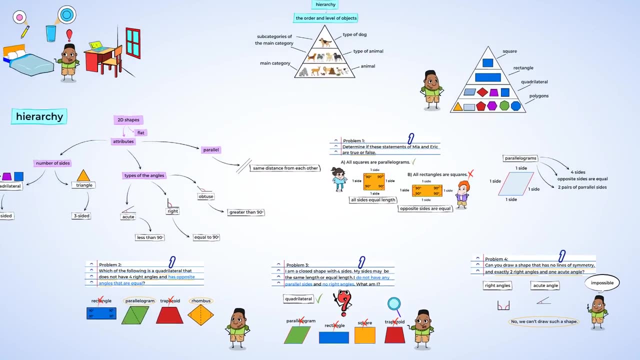 Wow, we did a great job working with shapes and their attributes today. Our math knowledge helped us to solve some great puzzles And I can't wait to solve more mighty problems with you in the next lesson. Thanks Will, Bye, Bye. Bye, Bye, Bye.